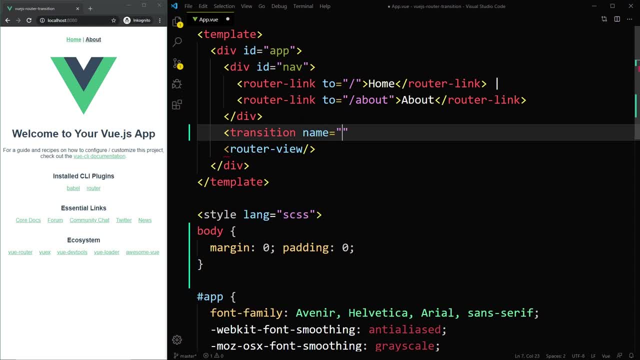 By Vuejs, and you can choose a name for your transition. it's totally up to you. I write here merely fade, And you can use several modes for your transition and in this case makes the out in mode sense, so that first the current page goes away and after that the new page fades in. 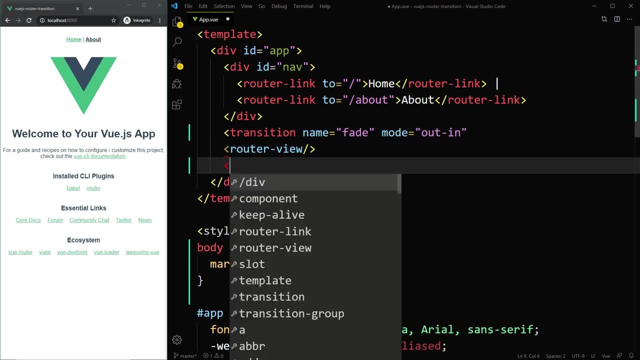 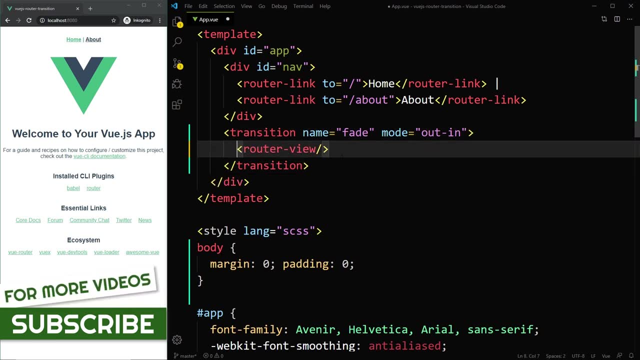 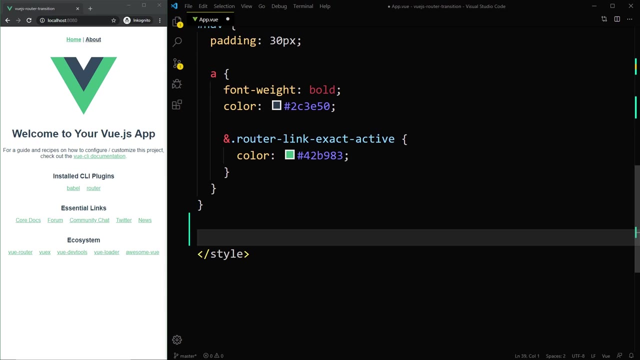 Last but not least, We should close the transition tag after the router-vue. Ok, we are done here in the template. let's go to the stylings. yes, we make a CSS transition And there are several predefined CSS classes you can use for this. each class is for a. 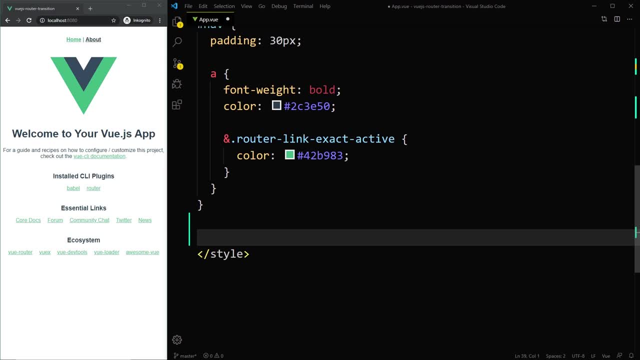 specific part of your transition where you can set your CSS definitions. The first we need is the enter class, but to match this class to our transition tag in the template we have to set a prefix, in this case the name from our transition fade. 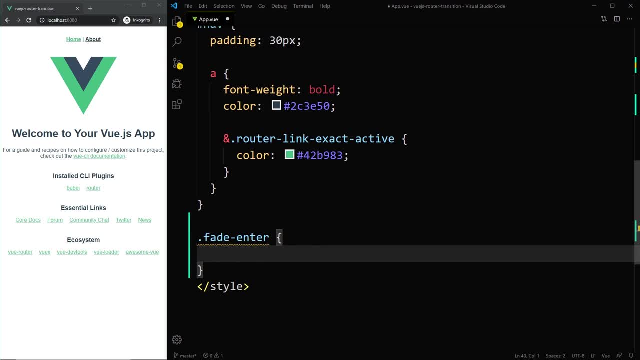 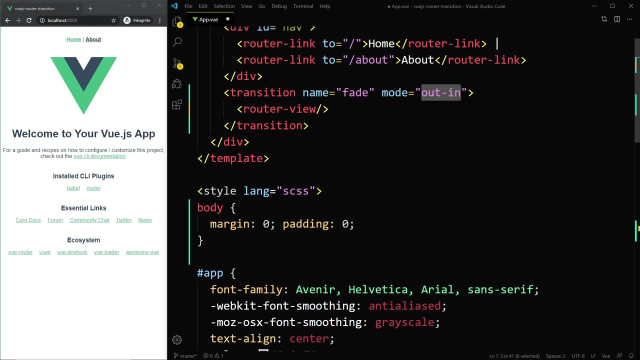 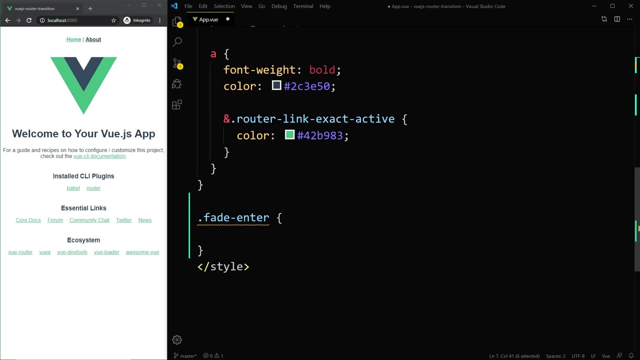 And this class is the starting point. but we have to think differently in this case. we use here the mode out in, So we have to define here the state Where the content is not visible. I do this with opacity and set it to 0.. 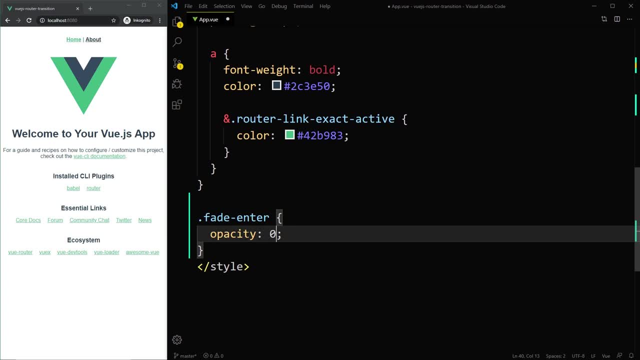 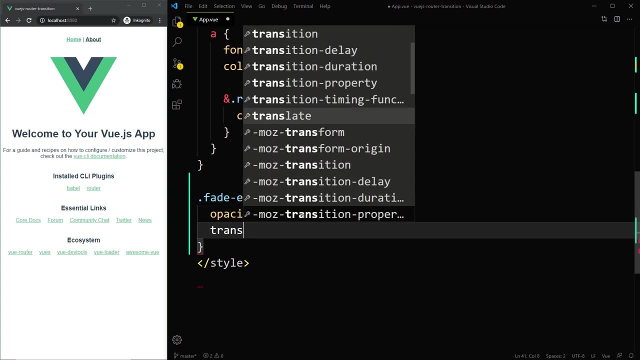 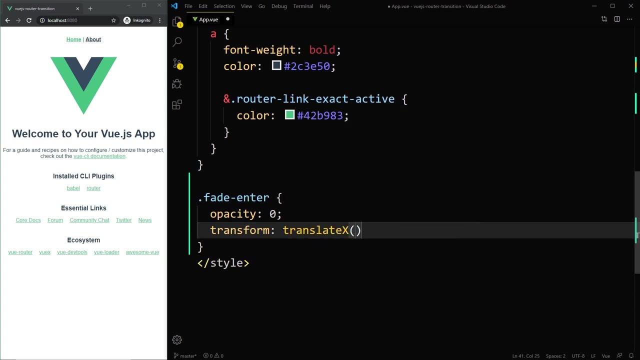 And I want to have a different position so that the content slides in from the right side. We can implement this with transform and translate x for the horizontal axis and as value maybe 2em. Ok, By the way, if you want it from the left side, so you can write here: minus 2em. 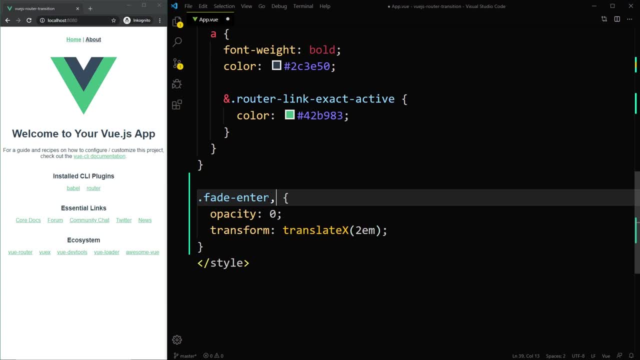 Ok, this should also be the same for the leave top class. so let's add this right here. And this class is for the end point from our transition, not from the enter transition here. that would make no sense. it's for the leave transition where the page goes away.